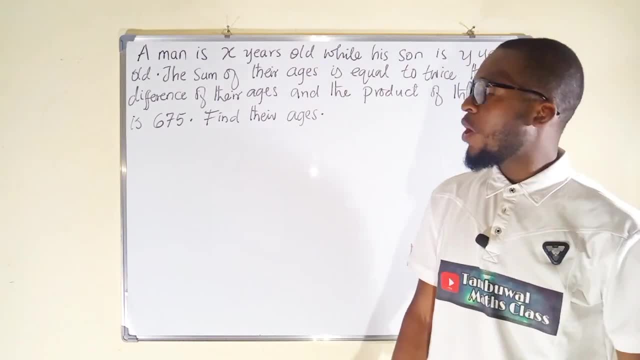 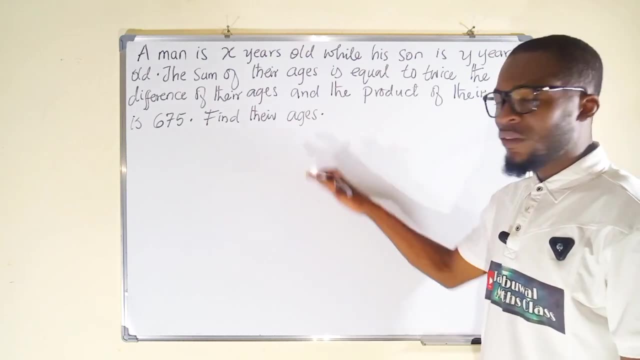 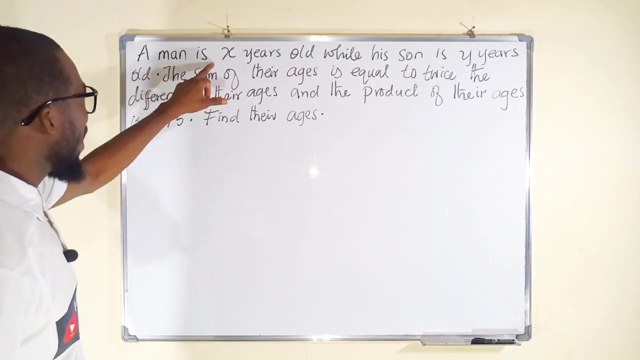 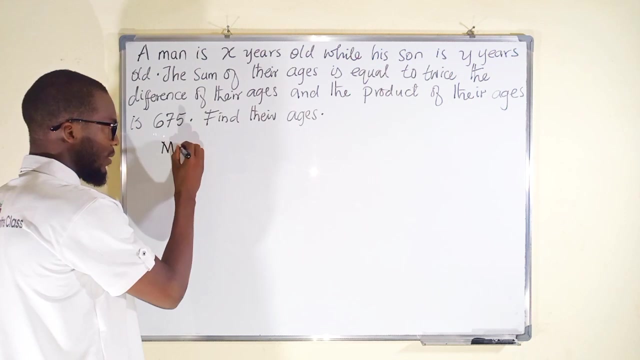 asked to find their respective ages. So how can we tackle this question? Okay, we are going to follow this question line after line and see how we can transform it into some equations. All right, A man is X years old, So the man has X years. His son is Y years old. The sum: 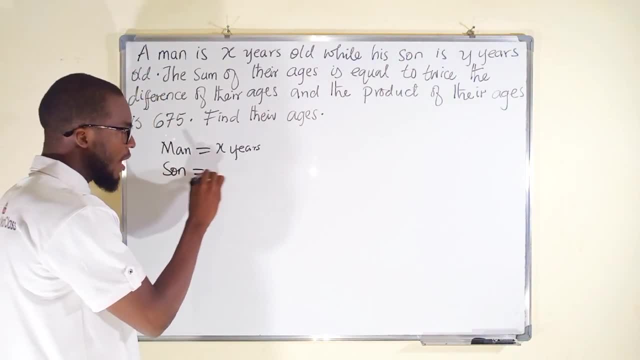 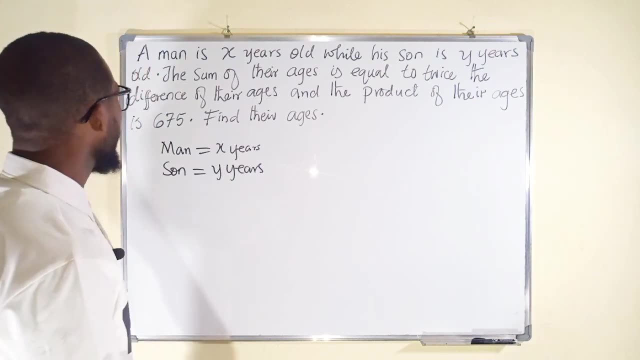 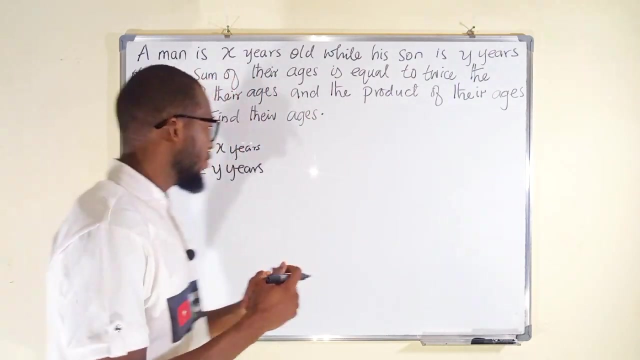 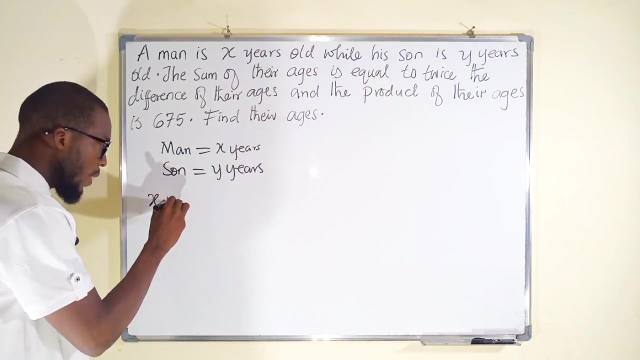 of their ages equals twice the difference of their ages. So how can we tackle this question? uh, has Y S We're going, but we learnt that the sum of their ages, sum meaning addition. So we are going to add their ages together before we continue in the question. So the ages will be X plus Y for the father and his son. So we meant saving zero to have the 4 for X. so we're going to use this sum and the sum would be several of them. The sum in thistel will be X plus Y, so that there will be. 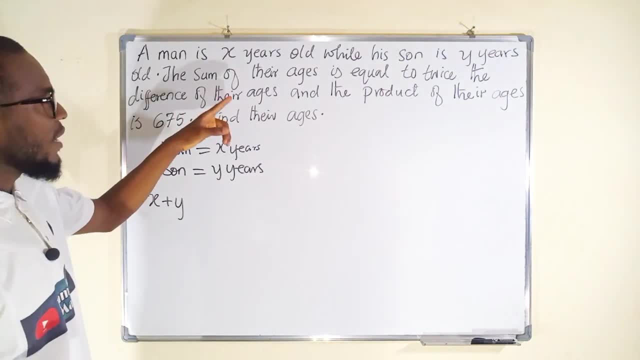 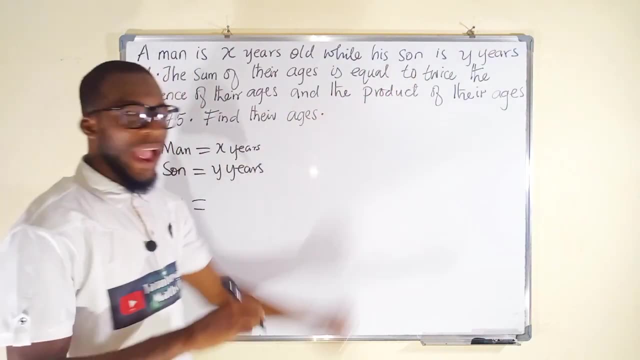 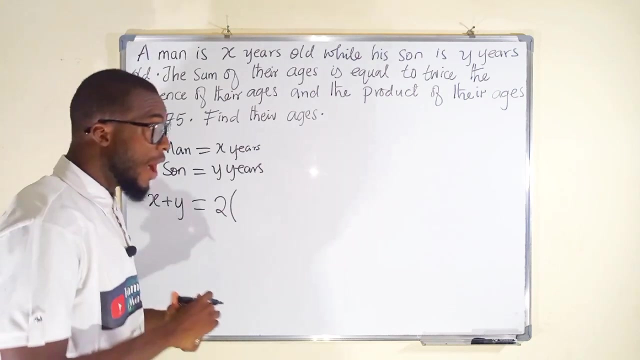 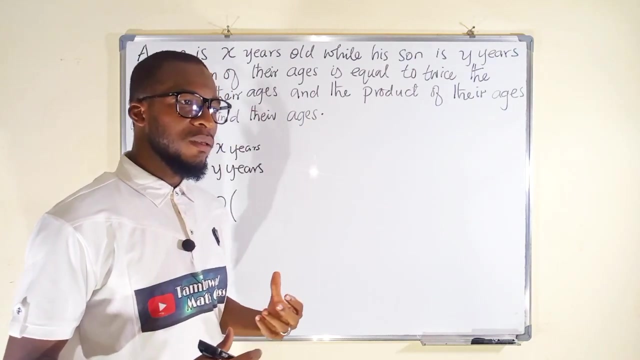 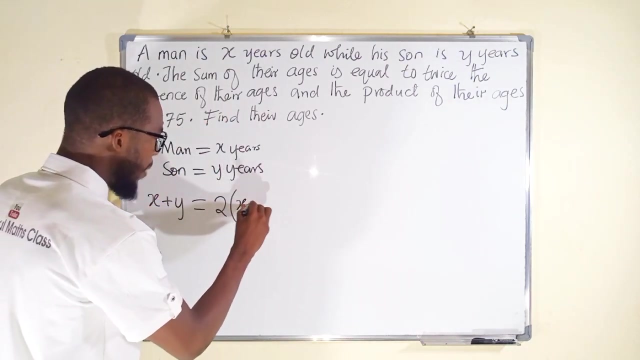 but after adding this ages together, we learned that it is going to be equal. okay, look at this: equal twice. whatever it is that is going to be twice double, twice the difference of their ages difference. definitely, you know that the father's age will be greater, so let's start with the palace age. we say x minus y because 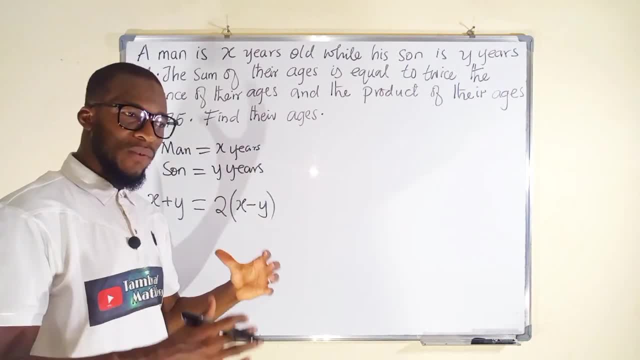 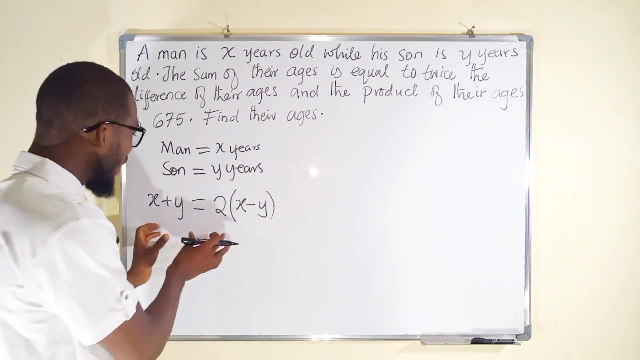 we are talking about difference. to find the difference of every two numbers is to subtract the smaller number from the bigger number. so right here we have formed an equation which we can expand this if we like. we can say: x plus y is equal to you distribute this. 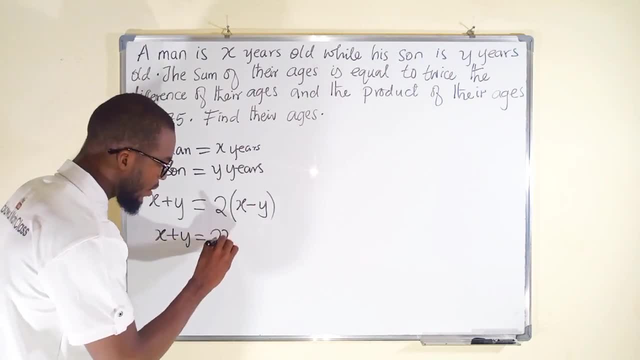 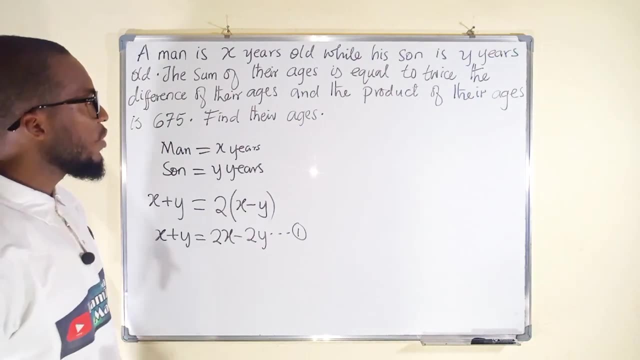 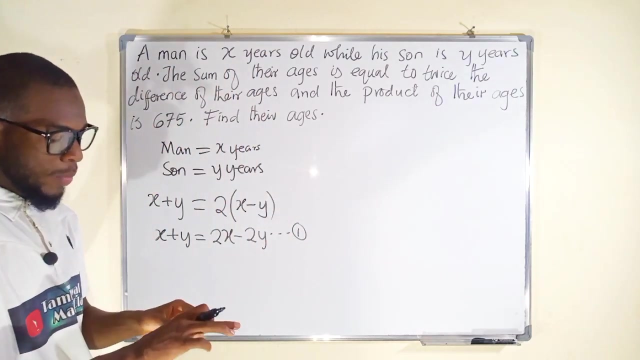 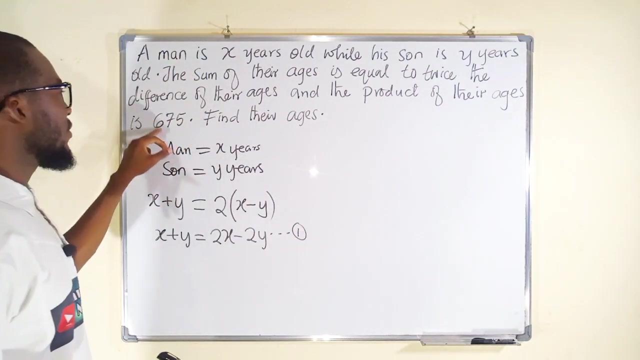 number into this parenthesis. we have 2x minus 2y and we can call this one equation one. then we continue reading the question. it says that the product of their ages is 675. product, you know, is multiplication. it means that if we multiply their ages together, we shall obtain 675 years, so x. 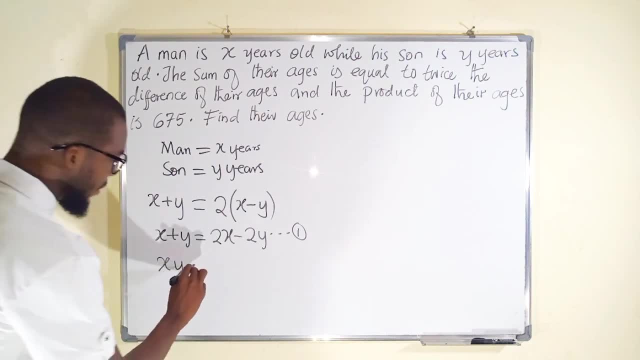 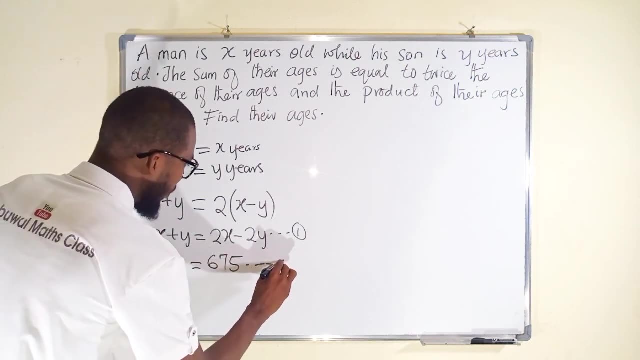 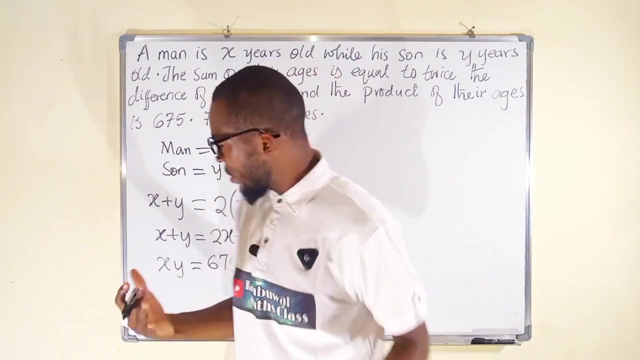 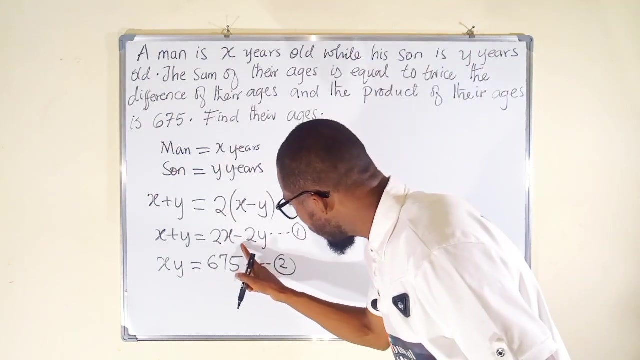 x multiplied by y, x, y is equal to 675. this is another equation. equation two: all right, now we have formed two equations. what do we do next? look at this equation one. we can bring the like times together. you can see this negative 2y. if you take it to the left, it becomes positive. 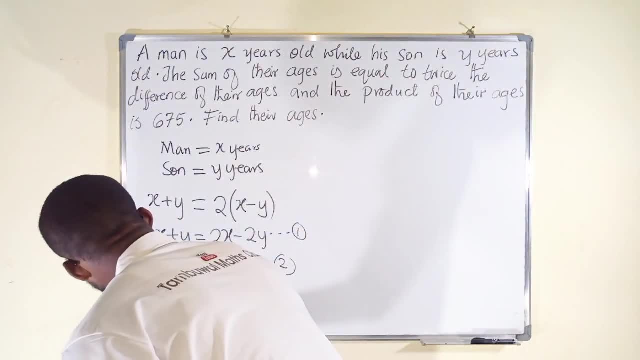 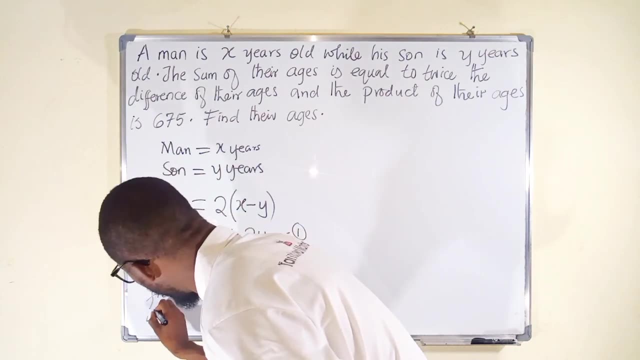 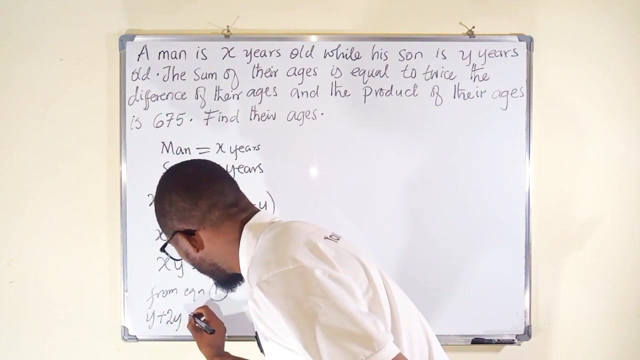 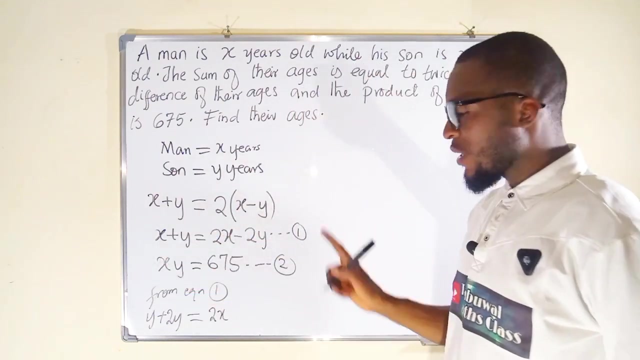 so we may have y. okay, let me write it from equation one. we can bring this backward. already we have y there. bringing negative 2y back, it becomes positive to y to the right. we already have 2x there. if you take x to the right, it becomes negative. so we have negative x. let's continue to the other side. 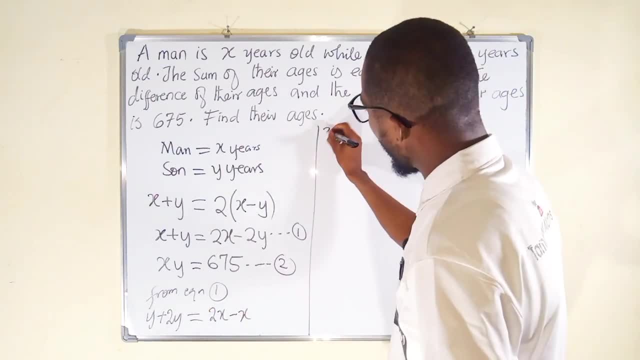 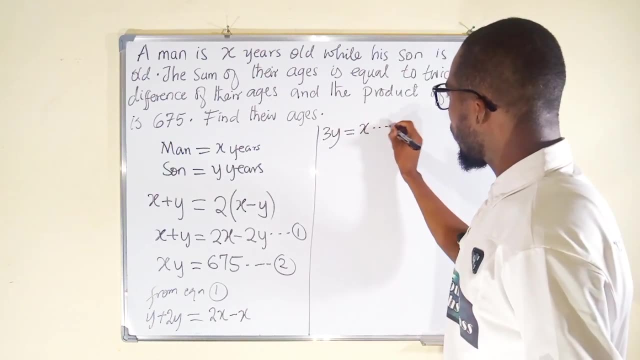 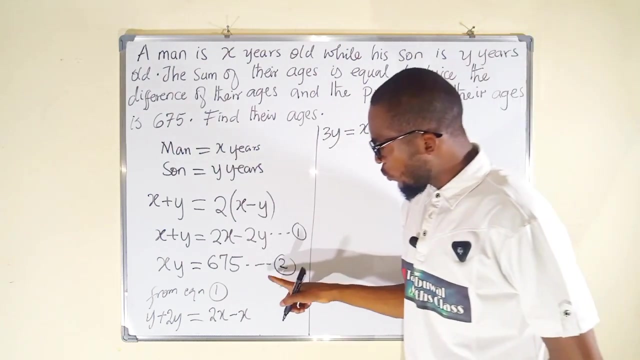 let's continue to the other side. let's continue to the other side. simplify this: we have three y's and to the right we have 2x minus x is just a single x. this is another equation formed from equation one. but from equation two we can see x multiplied by y. 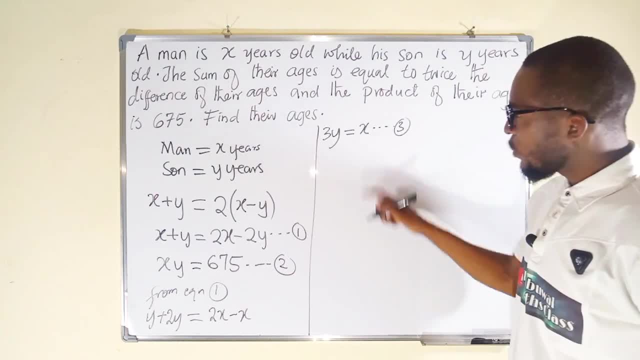 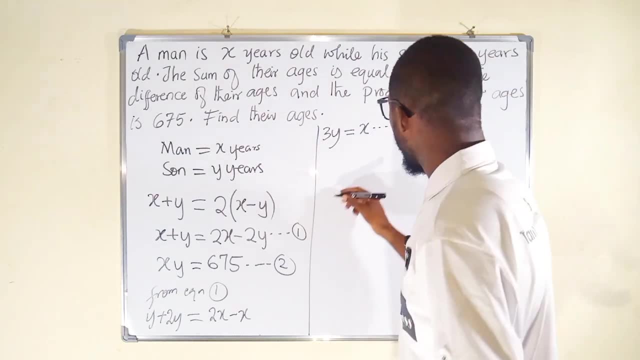 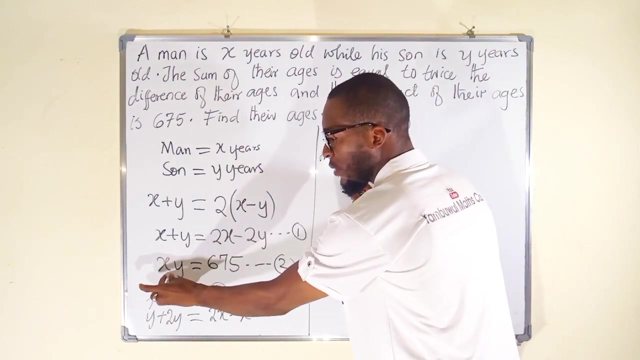 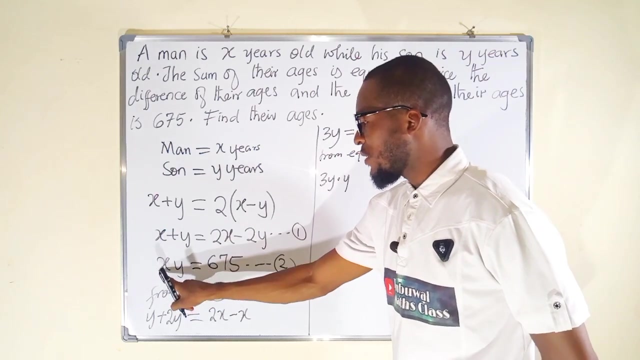 is exactly 675, so we can substitute the value of x in that equation as 3y. so wherever we see x, we replace it with three y. so you write from equation equation two: instead of writing x, y, you can write it as 3 y multiply by y, because you can see x is equal to 3 y here and we already. 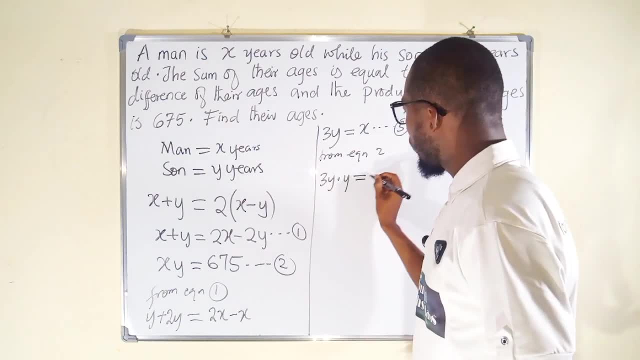 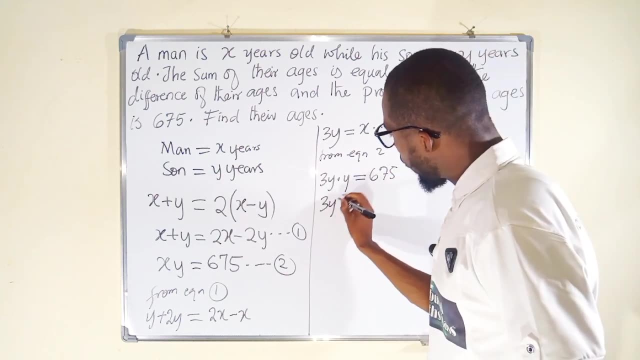 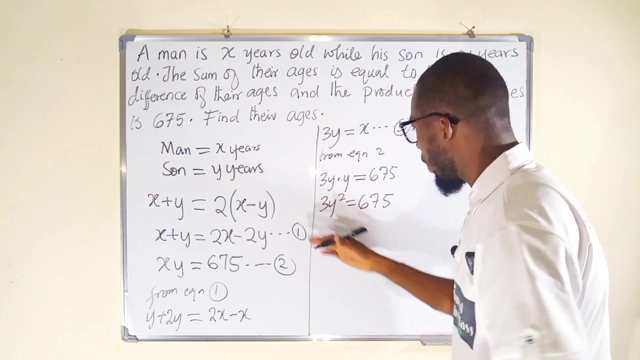 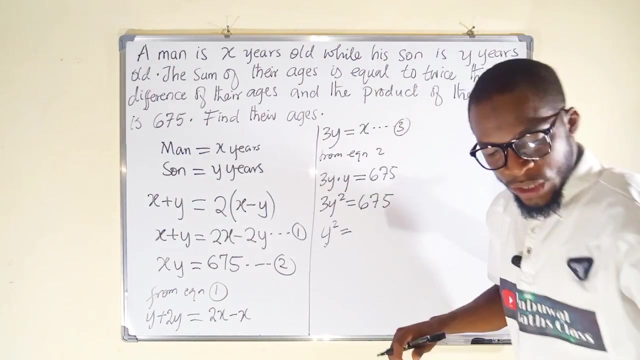 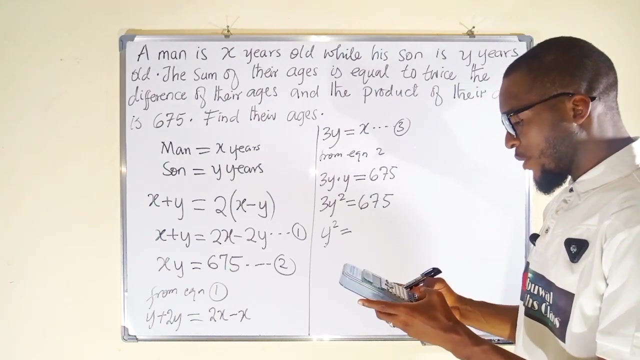 have y to the other side. then we multiply them together. all this will give us 675.. this becomes 3. y squared equals 675 to. to get rid of this coefficient, we can divide both side by that, so y squared will be equal to. let me divide this number by 3. we have 675 divided by 30, and. 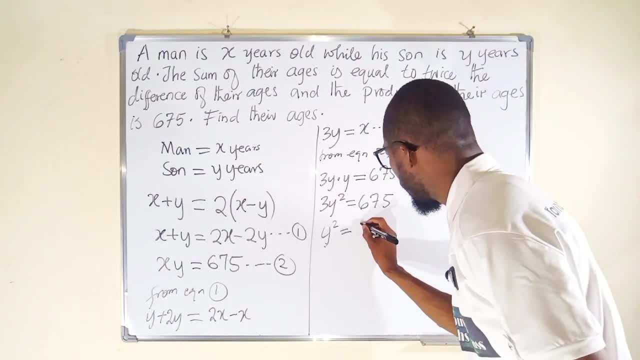 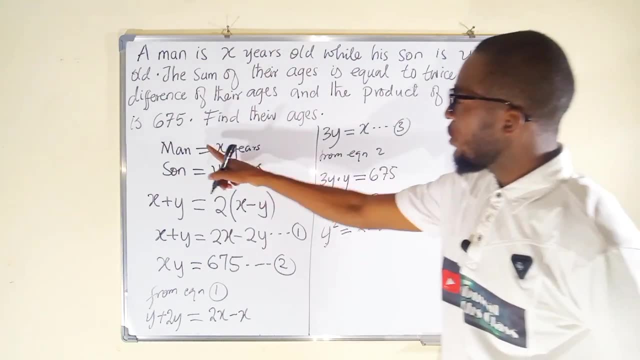 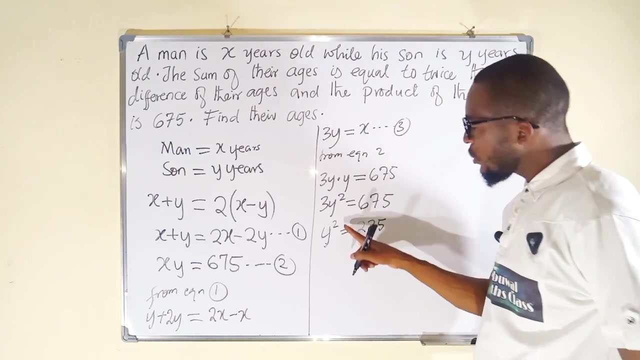 this gives us 225, so we have 275 and 25.. remember, y is that of the sun. we want to find his age. his age is not y, squared rather y. so we're going to take the square root of both sides to eliminate this power of two. 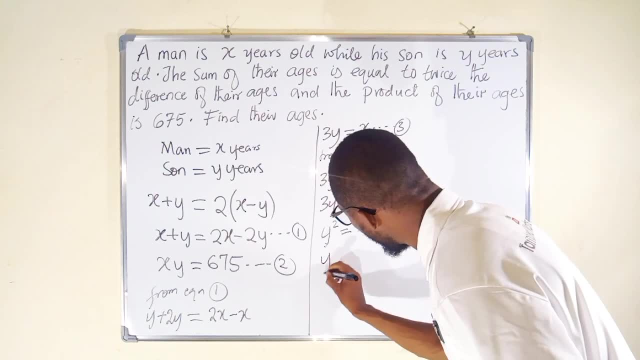 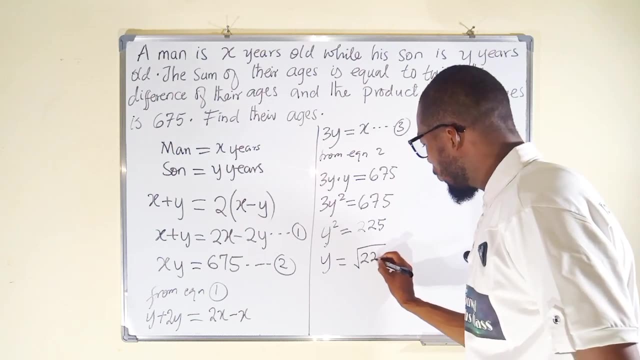 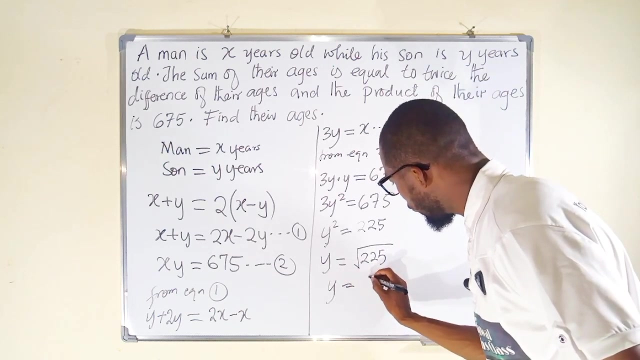 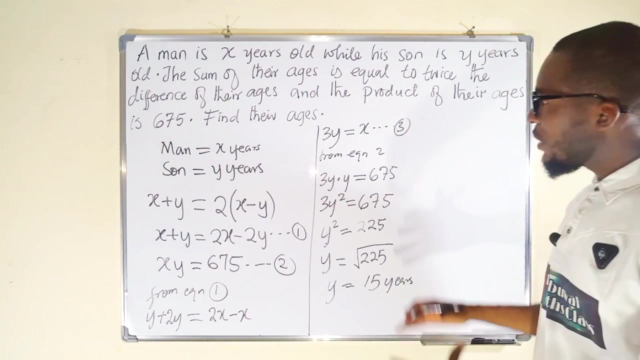 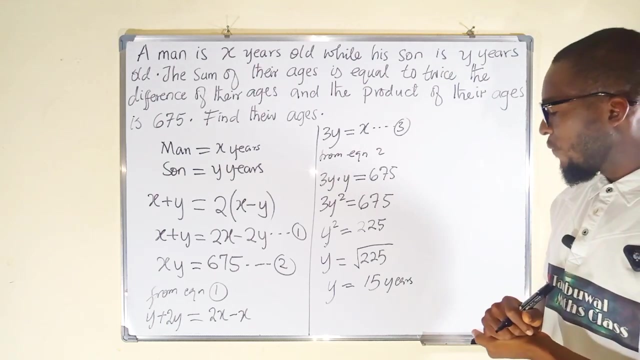 you know, normally we do used to add plus or minus, but this time around we are going to only consider the positive sign, because we do not have a negative h, only positive h. so y, finally, is equal to 15, and this 15 is in years. so you can see, the age of the sun is 15.. now let us go ahead and find the age of. 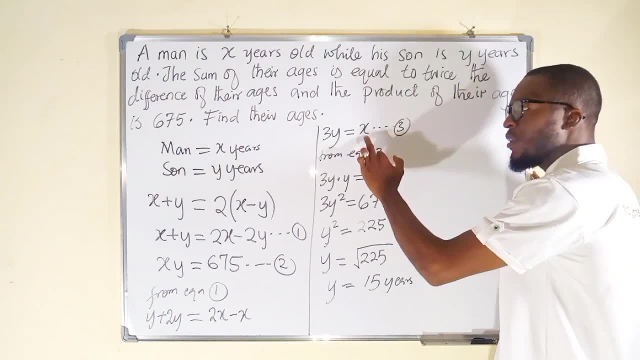 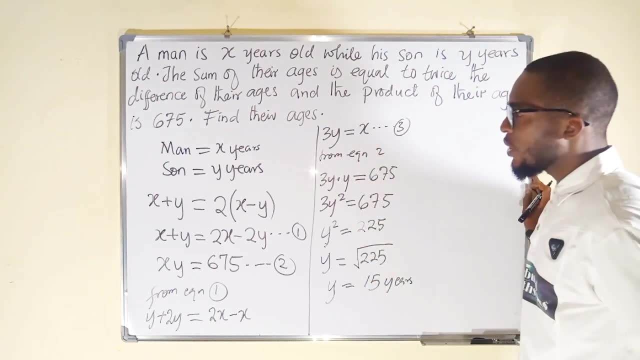 the father. which equation can we use? you can see, x represent the age of a father. so we can substitute this 15 in this equation to obtain the age of the father. so we can substitute this 15 in this equation to obtain the age of the father. 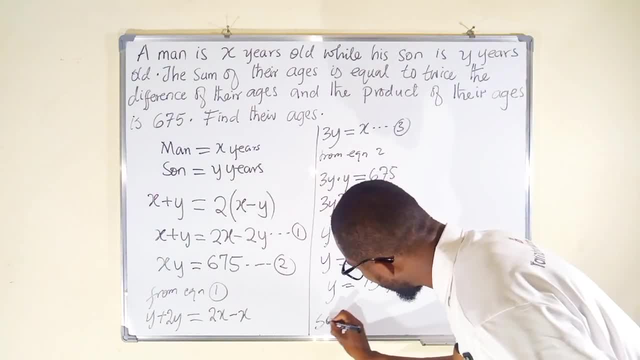 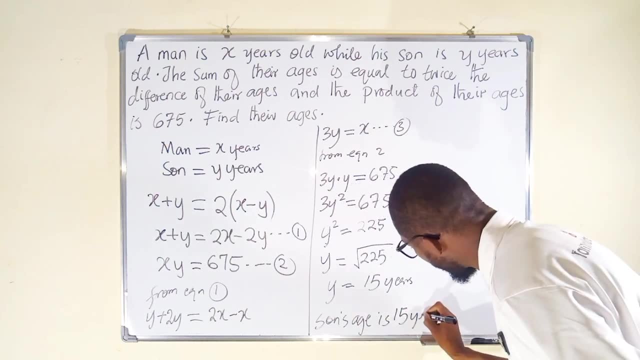 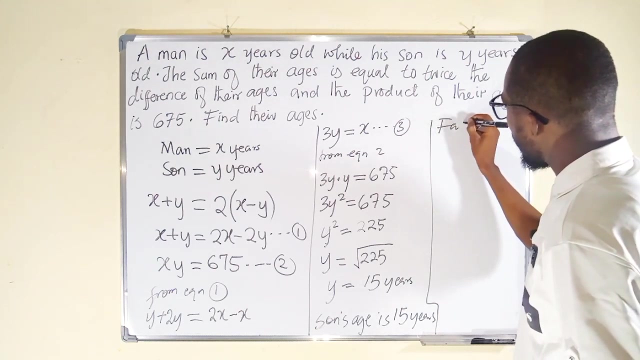 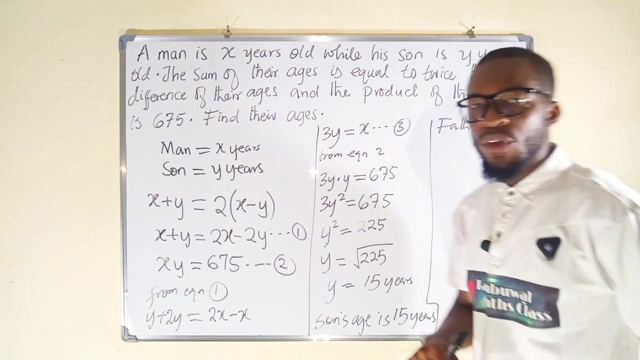 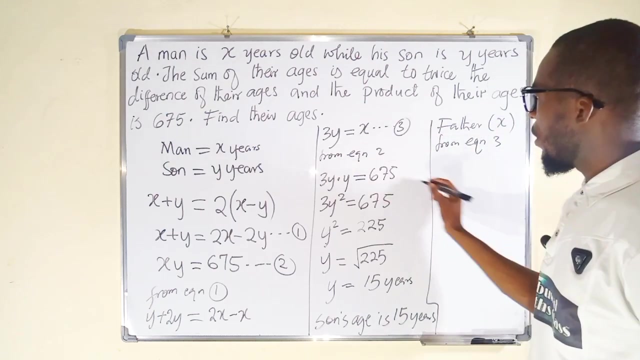 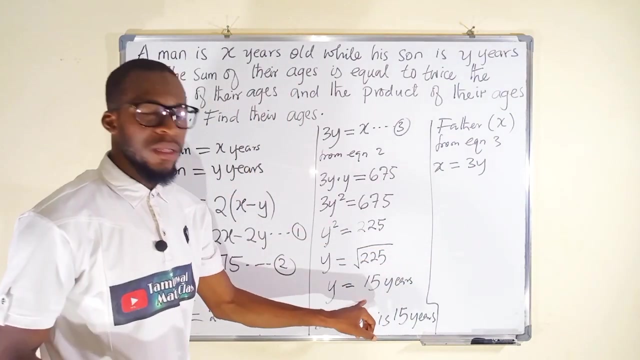 so this is for son. son's age is 15 years. so now let us go ahead and find that of the father for the father, the father, which is x. you can see it from equation 3. from equation 3, X will be equal to 3Y and Y is already 15, so we can say that X is equal to 3. 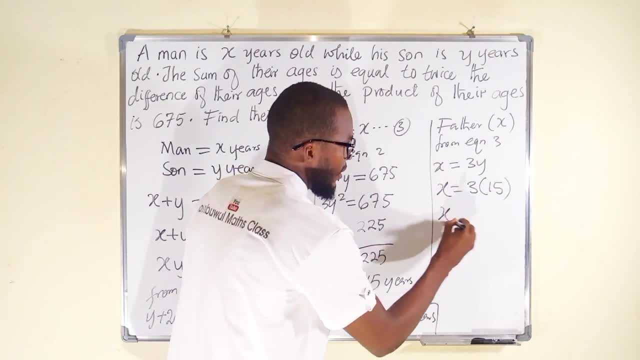 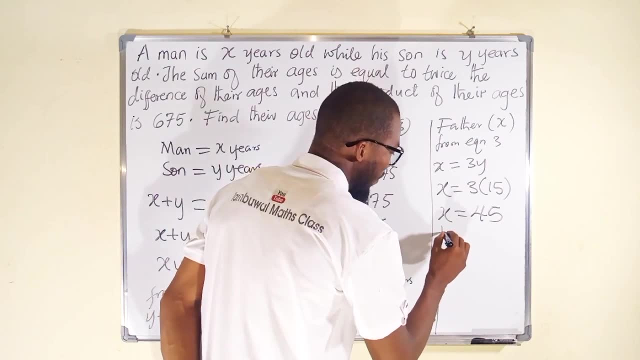 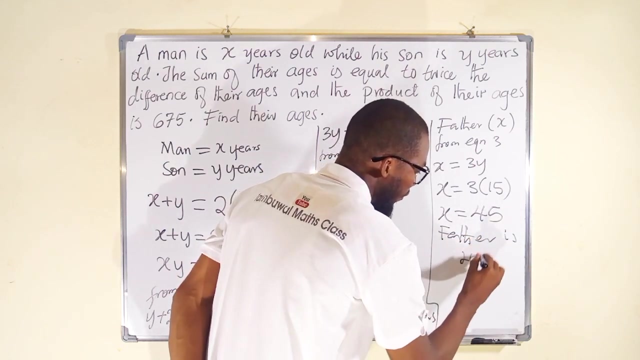 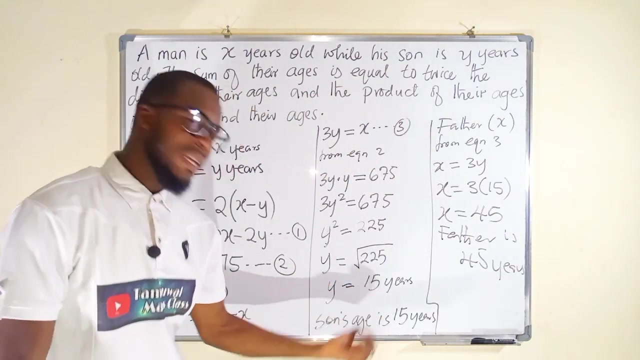 multiplied by 15, and X, finally, is equal to 3 multiplied by 15, which is 45, and hence the age of the father is 45 years. so you can see we have obtained their corresponding ages, for the son is 15 years and for the father is 45 years. now, 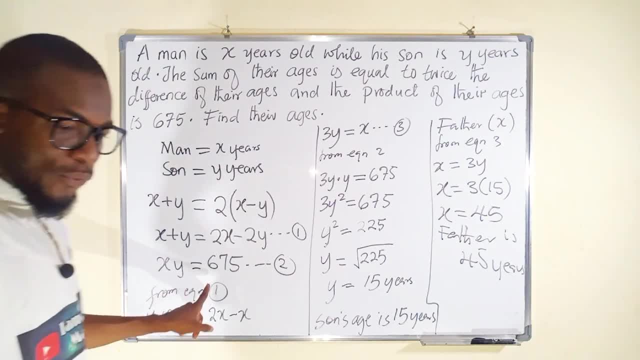 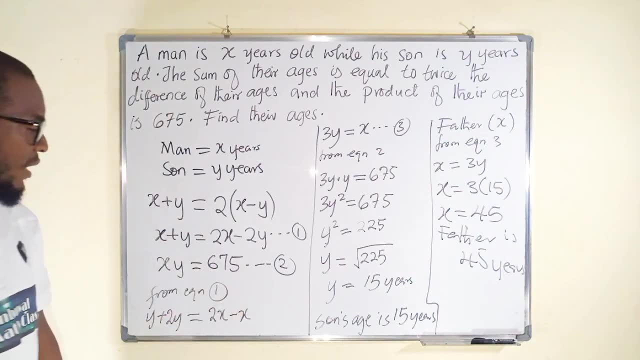 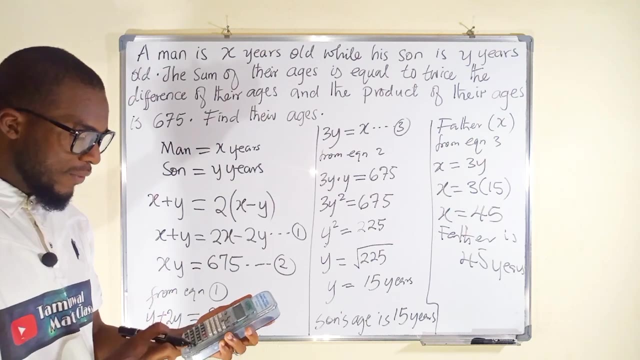 let us see whether this is true from this equation number two. it says that if you multiply the age of the father and that of the son, you shall of 10, six hundred and seventy five. so now I want to do that here: 15 x 4, 5 is exactly 675, which is true. and now we can tell the other one: he.